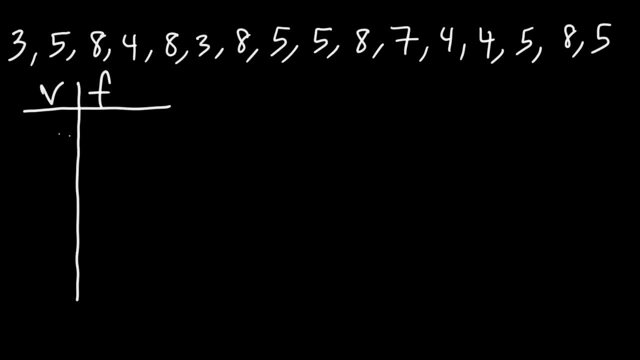 Let's start with the lowest value in our data set. The lowest value is 3.. Now how often does the number 3 appear in that data set? Notice that we could see it two times. So the frequency of that value is 2.. Now let's look for the next highest number. 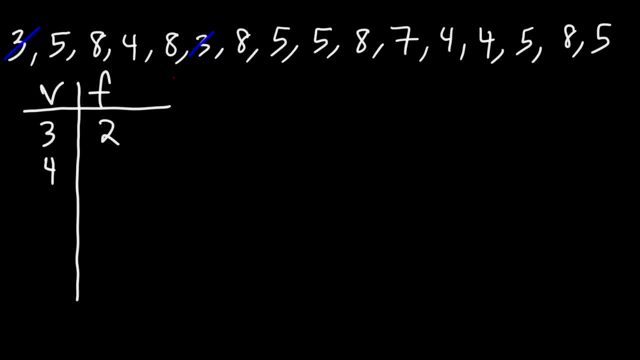 The next number in the list is 4.. And there are 1,, 2,, 3, 4s in our data set, So the number 4 has a frequency of 3.. Now let's move on to the next highest number. The next highest number is a 5.. 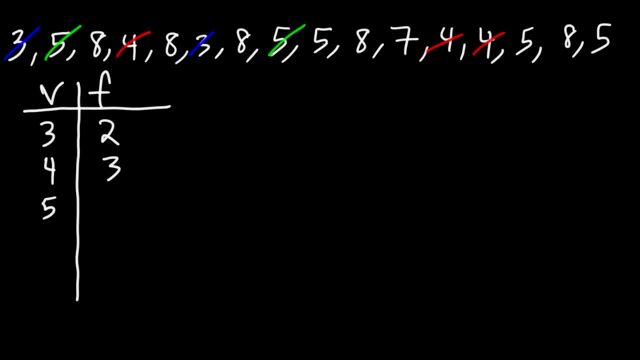 And so we have 1,, 2,, 3,, 4,, 5,, 5s- I believe I counted all of them. Now the next highest value is a 7.. So we only have one 7 in our data set. 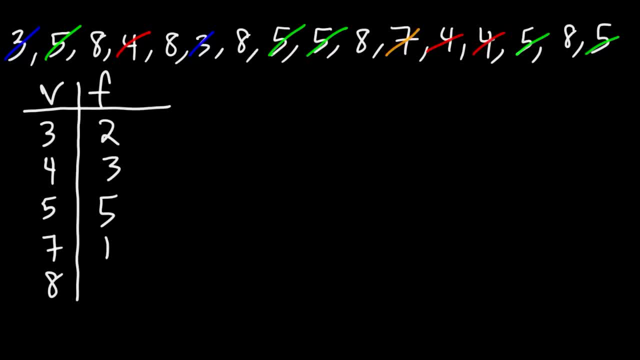 Next is an 8.. And I could see 1,, 2,, 3,, 4,, 5, 8s, So that's a very simple way to make a frequency table. Now, how can we use this table to calculate the mean, the median, the mode and the range? 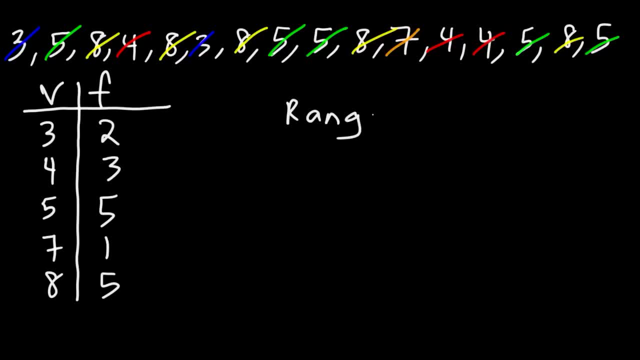 Well, let's start with the range. The range is the difference between the highest number and the lowest number, And so we can see that the number with the highest value is 8.. The number with the lowest value is 3.. So, in this example, the range is going to be 5 minus 3.. 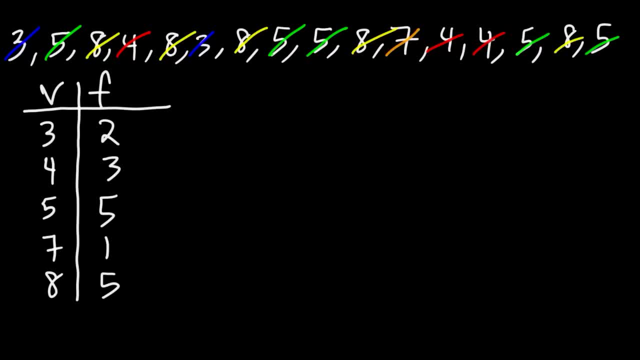 Now, what about the mode? How can we use the frequency table to calculate the mode? The mode is basically the number in the data set with the highest frequency. So in this case there's two such numbers, Because the highest frequency is 5.. 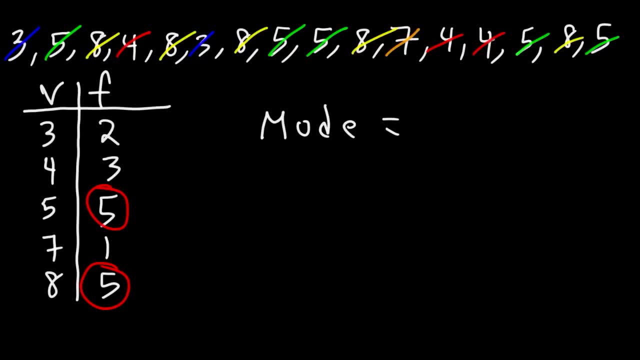 So the range is going to be a bimodal data set, meaning that it has two modes. The value of the first one is 5, and the value of the second mode is 8.. Now let's say, if we introduce another number, 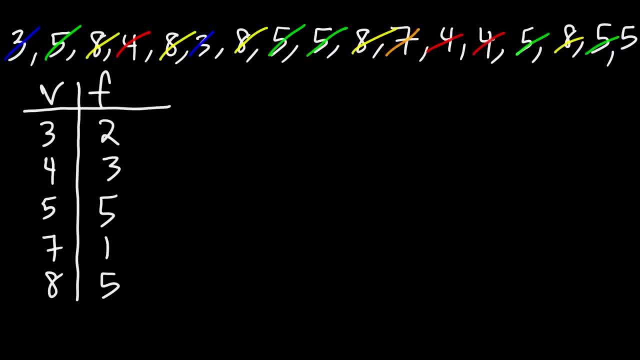 Let's put another 5 here, So the range is not going to change. So now we have a total of 6 5s instead of 5 of them. So in this case the range is not going to change. So now we have a total of 6 5s instead of 5 of them. 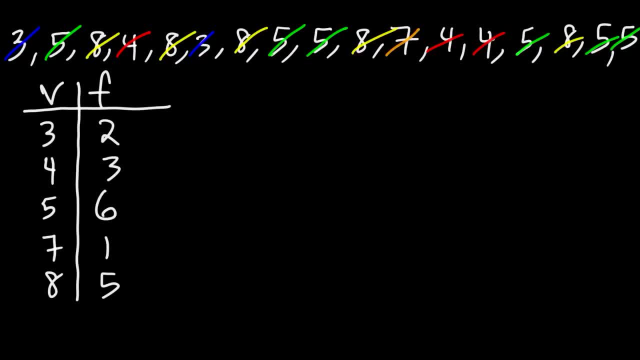 So in this case the range is not going to change. It's no longer a bimodal data set, It's a unimodal data set, So there's going to be one mode. Since now 5 has the highest frequency, the value 5 is the mode of the data set now. 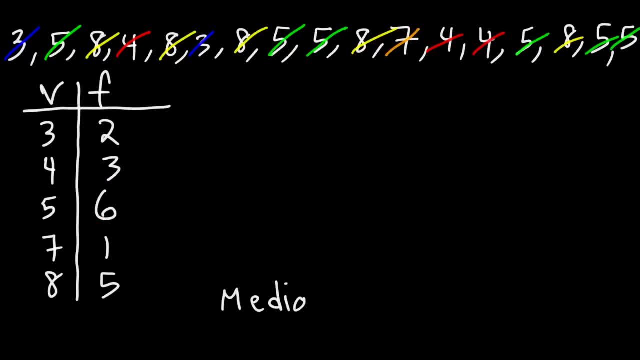 Now let's calculate the median. The median is basically the middle number in the data set, if it's arranged in increasing order. So how can we use the frequency table to determine the median? So notice that we have the first 5 numbers on the left and the first 5 numbers on the right. 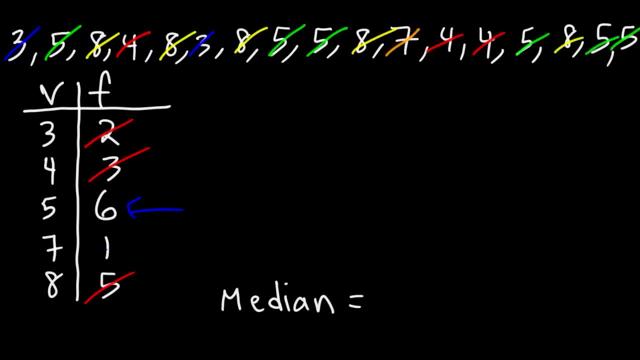 If we follow this pattern, it is clear that the middle number is going to be a 5.. So that's a quick and simple way to use the table. Now, if that confuses you, what you could do is you could write these numbers in ascending order. 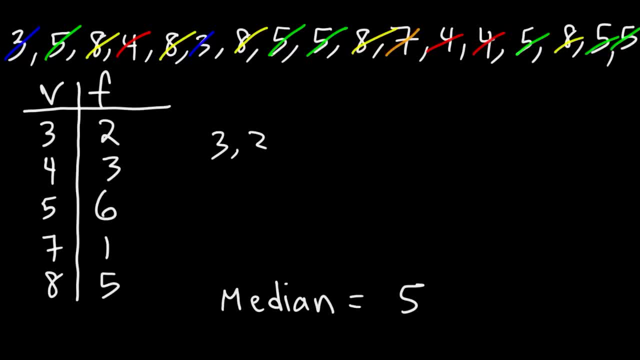 So we have two 3s, We have three 4s, We have six 5s, One 7. And eight 5s. So let's say we cross out the first 5 numbers on the left and the first 5 numbers on the right. 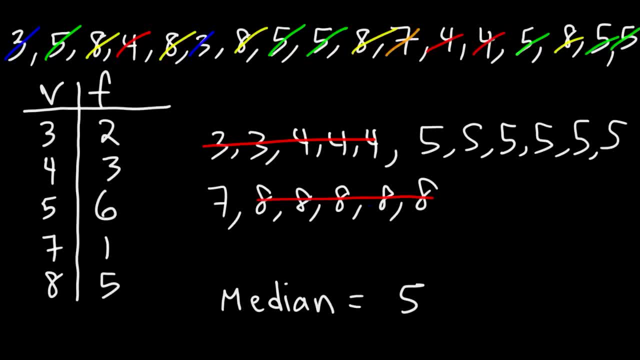 Next, let's cross out the next two numbers on the left and the next two numbers on the right And then let's repeat this pattern. So we have two 3s And then let's repeat this pattern, And so we can see that the middle number is 5.. 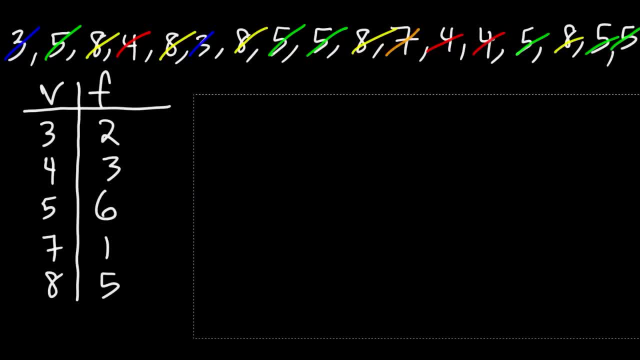 So that's the median. Now what about the mean, The average? How can we calculate the mean? in this example, The mean is basically the sum of all the numbers divided by the number of data items in our set Subtitles by the Amaraorg community. 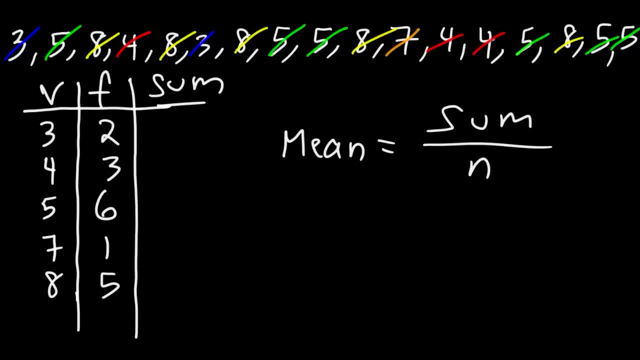 get our n value, what we need to do is basically add up all the numbers in the frequency column. so let's go ahead and do that. 2 plus 3 is 5 plus 6, that's 11 plus 1 is 12 plus 5 is 17. now let's calculate the sum we can multiply the. 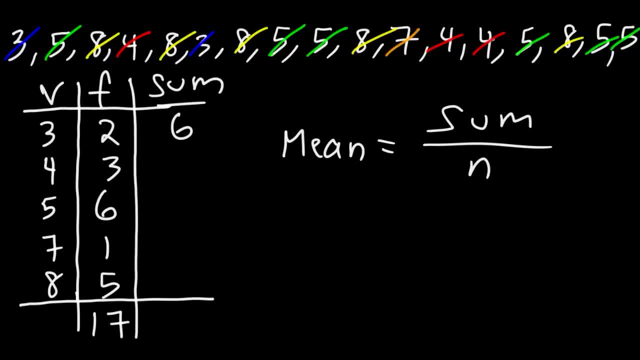 value by the frequency. so 3 times 2 is 6. we had two threes, so we're basically summing those two threes. 4 times 3 is 12, so this gives us the sum of these three numbers. and then 5 times 6 is 30, so that's basically the sum of the 5- 6. 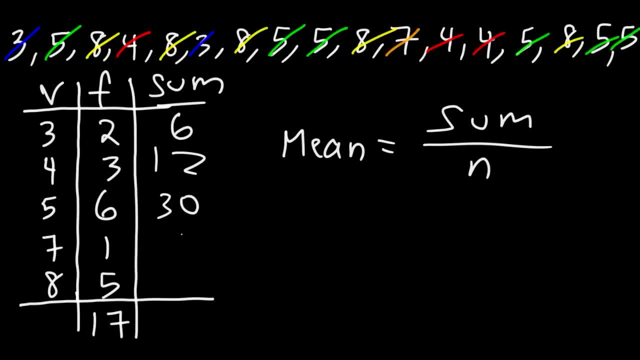 that we see in green. 7 times 1 is 7, 8 times 5 is 40. so now let's add up all the numbers in that column so we have 6 plus 12, that's 18 plus 30, that's 48 plus 755 plus 40, so it's 95. so 95 is the total. 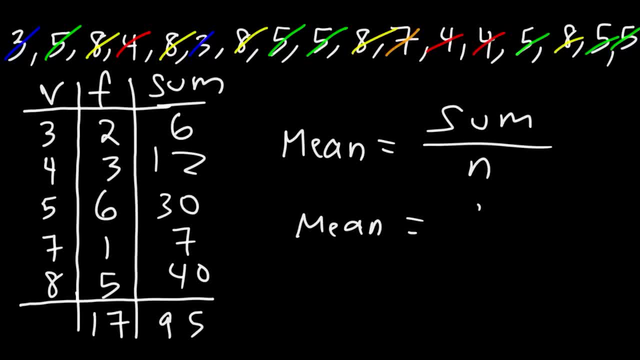 sum of all the numbers in the set, and there's 17 numbers. so 95 divided by 17, that's going to give us a mean of approximately. this is going to be our rounded answer: five point five nine, and so that's how you can calculate the mean, using a frequency table for the 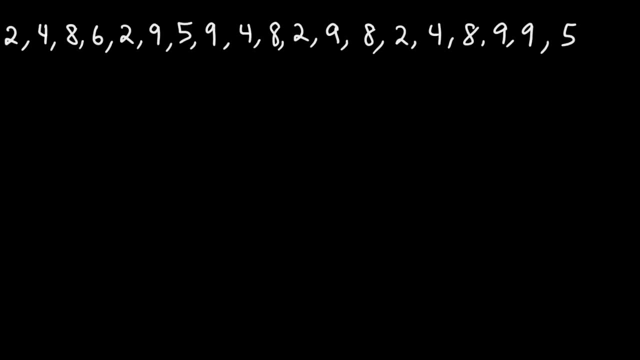 sake of practice, let's work on another problem. so pause the video and then use the data that you see here to make a frequency table. now, once you have that table, use it to calculate the mean median mode and range. so go ahead and try it. let's begin, let's start, with a two column table. so 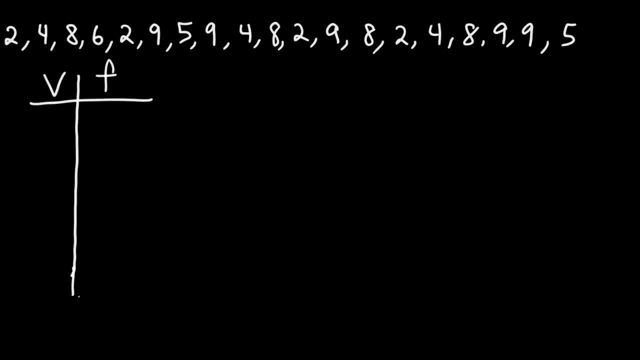 v for value, f for frequency. so the lowest value that we have is a two, and there's one, two, three, four, twos. the next highest value is a four, and there's one, two, three, fours. next up is a five, and so we have one, two, fives. 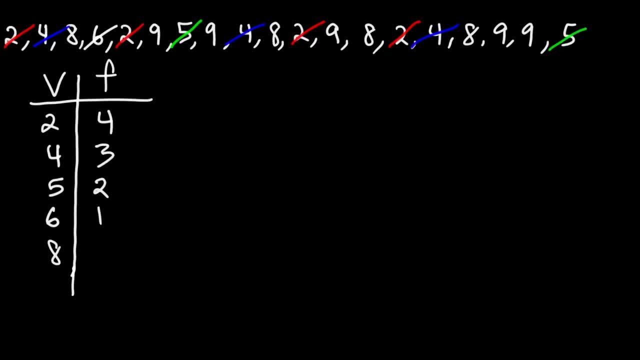 now there's only one, six. next we have an eight- let me use a different color- one, two, three. there's a total of four eighths and the highest value is a nine. so we have one, one, two, three, four, five, nines. so this is our simplified frequency table. next let's calculate the range. 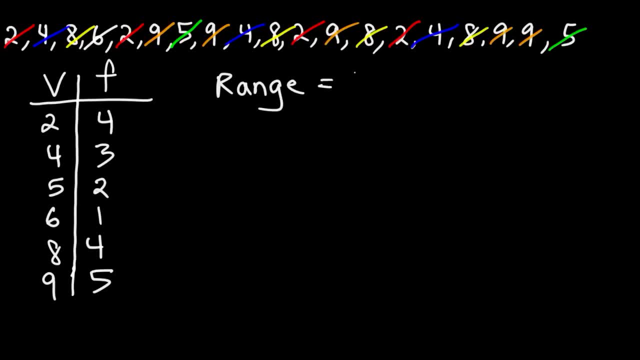 so, as we said before, the range is going to be the difference between the highest value and the lowest value, and we can easily see the highest value in our table. the highest value is nine and the lowest value is two. so nine minus two is seven. so that's going to be the range for this example. next let's calculate the. 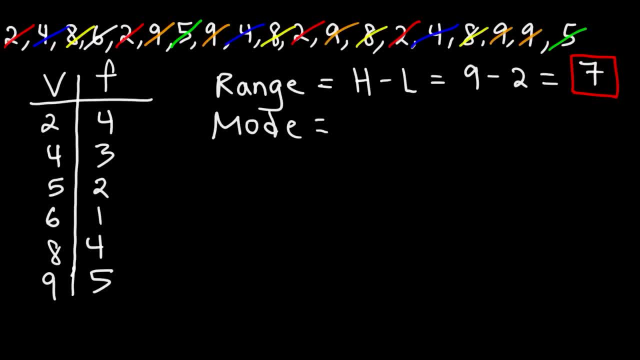 mode. as we mentioned before, the mode is the number with the highest frequency, and so five is the highest frequency. the value that corresponds to five is a nine, so the mode is nine. now, what is the median in this example? what is the middle number? what would you say? well, we could eliminate four numbers on the left side. 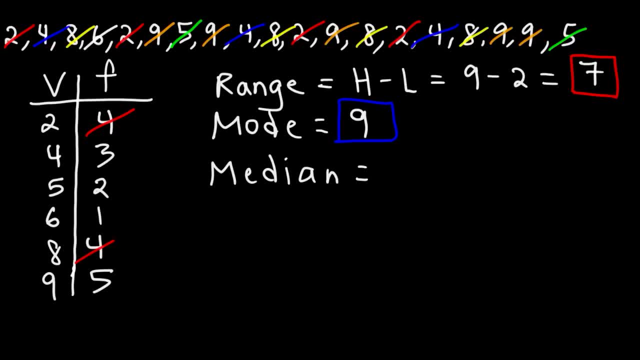 and four numbers on the right side. and then we can also eliminate five numbers on the left and five on the right, which means the middle number is going to be a value of six. six is the median in this case. now, if you want to prove it, let's write out the numbers in ascending order. so we have four twos. 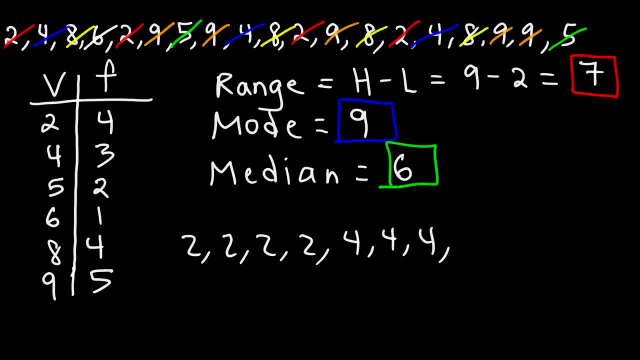 three fours, two fives, one six, four eights and five nines. so we can eliminate the five nines with four twos and one four. we can eliminate the next four numbers on the right side and the next four numbers on the left, leaving six as the middle number. so that's how.